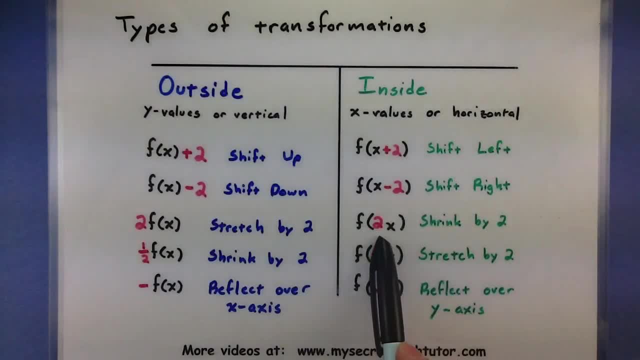 as what you think they should. So if you multiply by one on the outside, this will stretch it vertically, so it makes it look taller and smaller. If you multiply on the inside of a function by a number larger than one, then it will actually shrink it horizontally If you multiply on the inside. 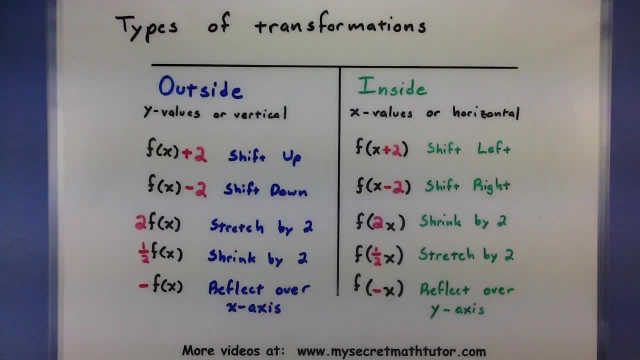 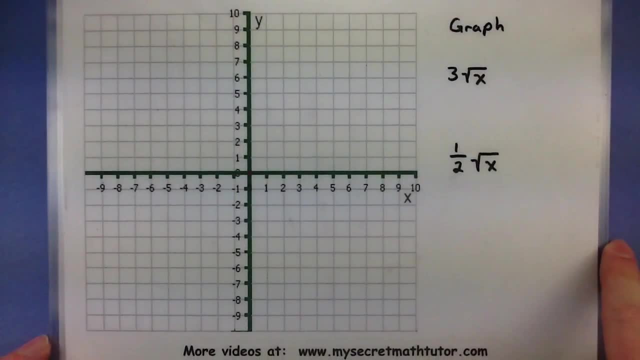 by a number between zero and one, then it will actually stretch it horizontally. We'll see this in our examples so you can get an idea of all of these different transformations. So let's start off with this guy. We want a graph: 3 times the square root of x and 1. 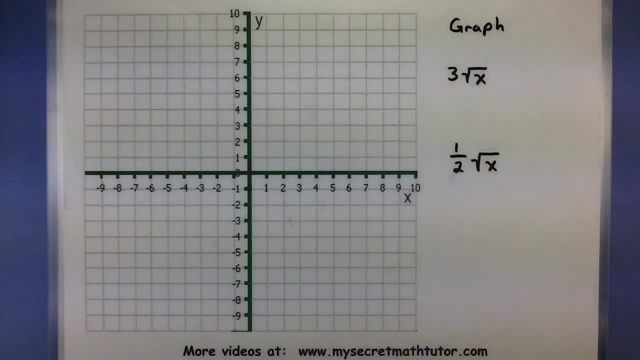 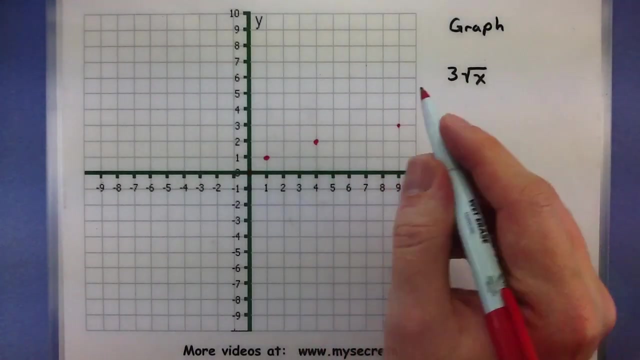 times the square root of x. Both of these examples involve our square root, so let's first graph that and start using it as our parent function. So I know the square root goes through 0,, 0,, 1,, 4,, 2, and 9, 3.. So we can consider this our parent function, Not. 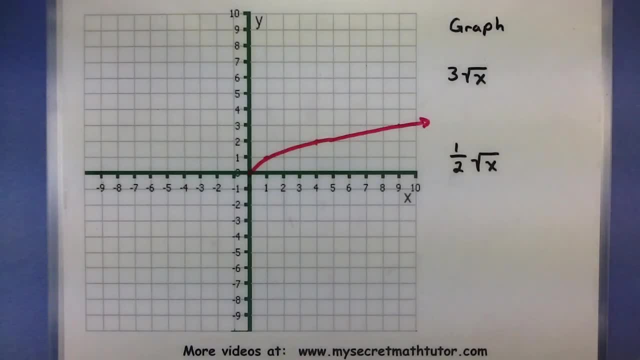 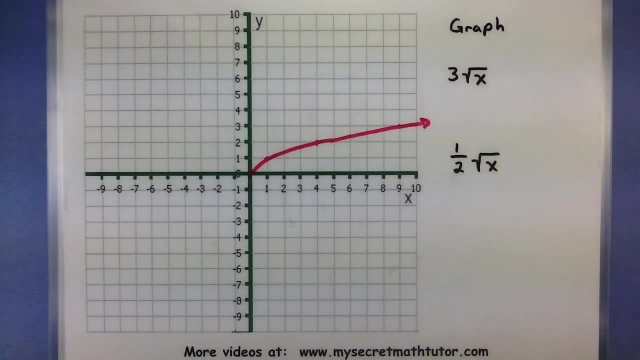 too bad, Alright. in our first example, notice how we are multiplying on the outside, So this will stretch it vertically by a factor of 3.. Here's how you can figure out where the new function is going to be. You want to keep track of these key points on the original. 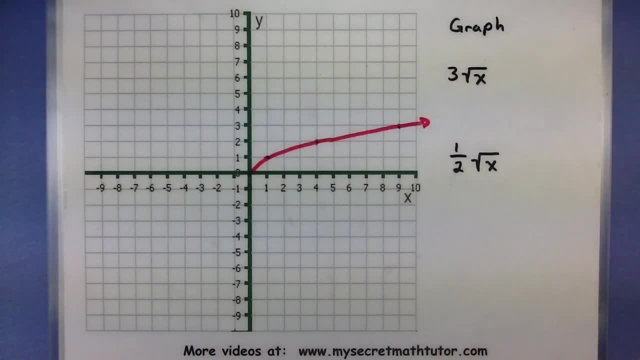 function and their y values. So you'll take all of those y values and multiply them by 3.. Let's start at 0, 0.. Now the y value here is 0, 0 multiplied by 3 is still 0, so we'll put that in the same. 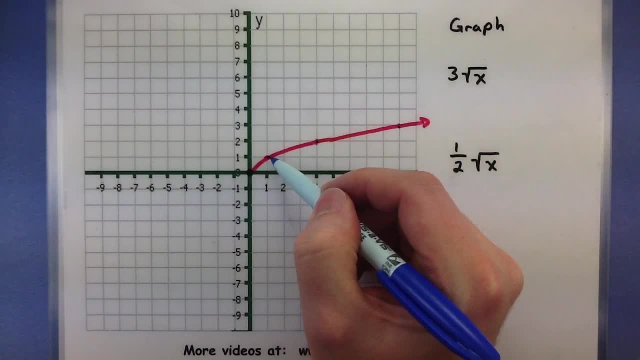 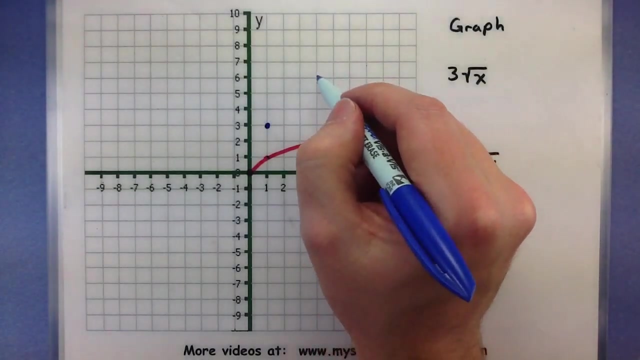 spot. Moving on, The y value here is 1, 1 multiplied by 3 is 3, so we're going to put that at one, 3.. The y value here is 2, 2 multiplied by 3 is 6, so we'll move that guy up to 6.. 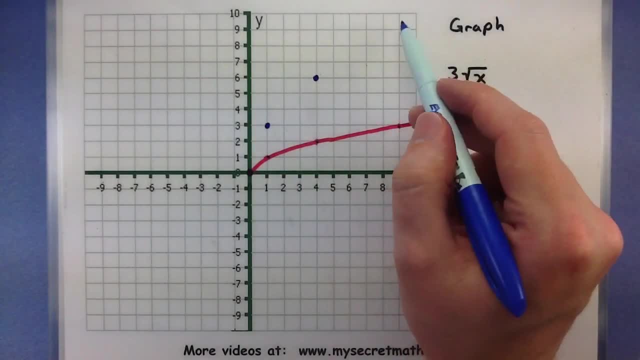 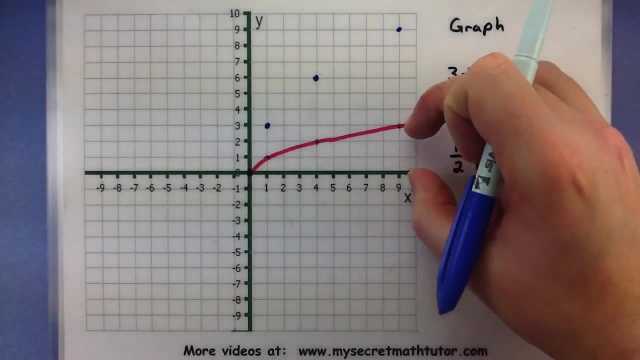 And lastly, the y value here is 3,, 3 times 3.. 5 times 3 is 3.. times 3 is 9.. So every single y value has been multiplied by 3.. Well, you want to see. 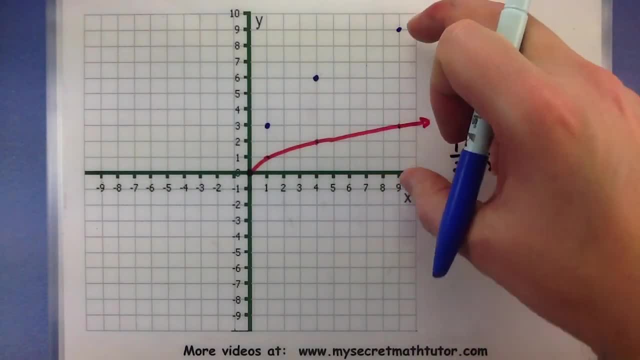 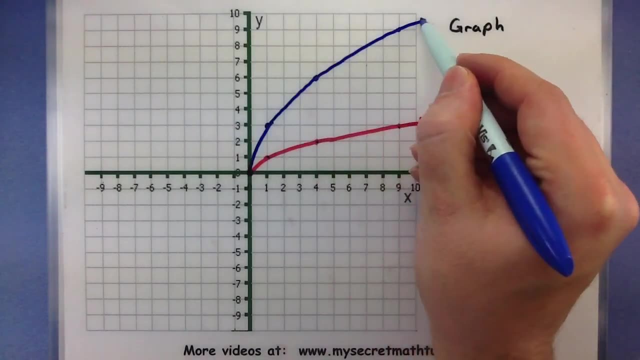 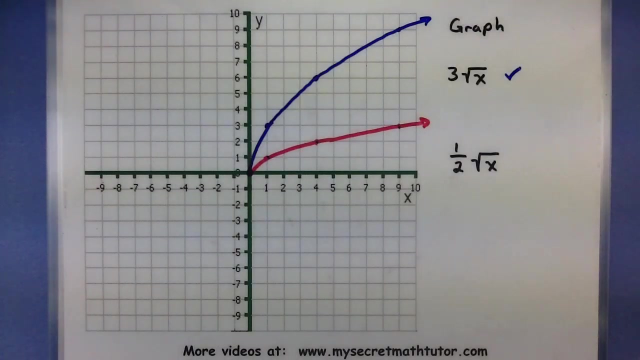 that each point is now 3 times farther away than what it used to be. Let's draw this guy in here. So you can definitely see that this graph has been stretched out vertically and it looks definitely taller than what it used to. Now let's multiply on the outside by a number. 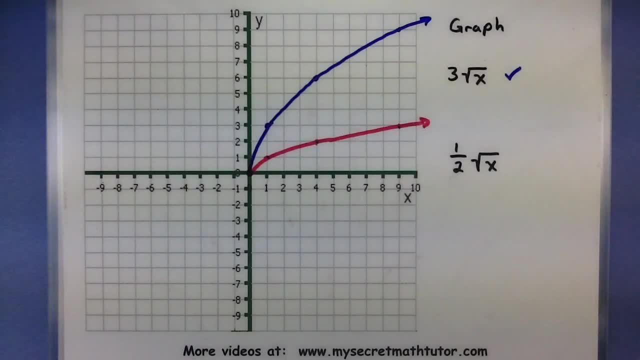 between 0 and 1.. So 1 half is a good candidate. We'll do the same thing. We'll take all of the y values and we'll multiply them by this 1 half. So 0 times 1 half starts at the same spot 1 times. 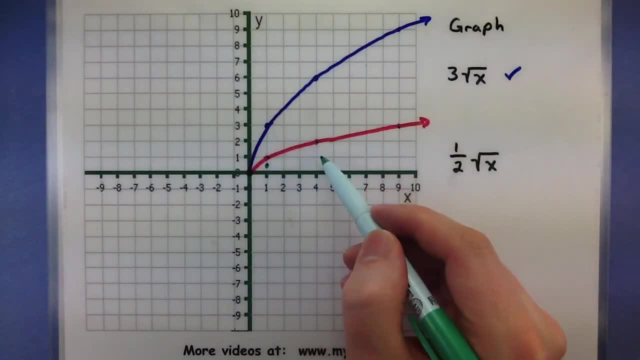 1 half is 1 half. 2 times 1 half is 1.. And 3 times 1 half 1 and a half. So this will make it a little bit easier to see. So let's draw this guy in here. So let's draw this guy in here. 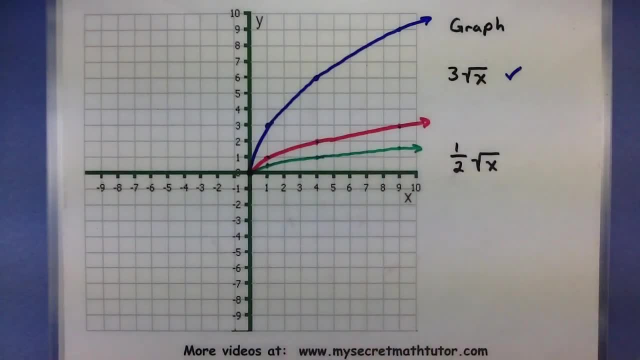 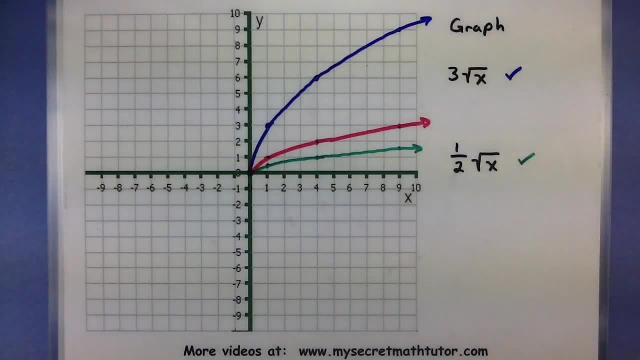 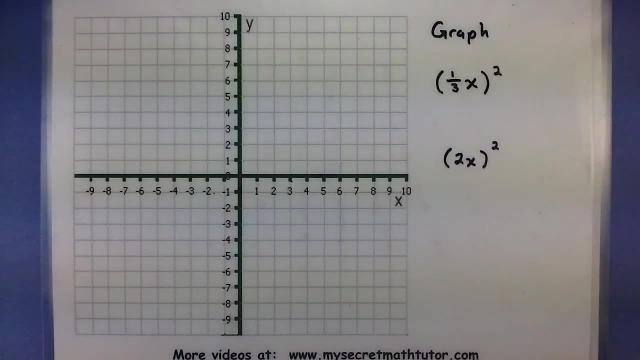 and we shrunk it vertically. Let's do this again with some more transformations, get a new function, try this all again. So this one I want to graph 1, third, x- quantity squared and 2x- quantity squared, since both of these involve squaring. I 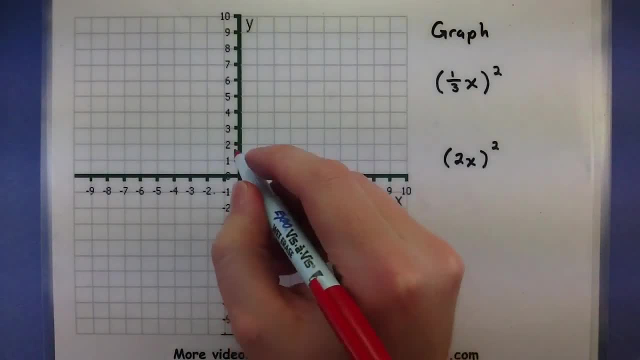 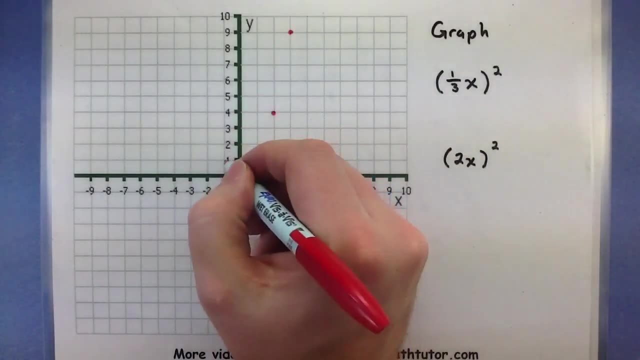 will start with my x squared as my parent function: 0, 0, 1, 1, 2, 4, 3, 9. now we got those same points over here: 2 forward negative 3, 9- bad. this will produce the familiar parabola shape. 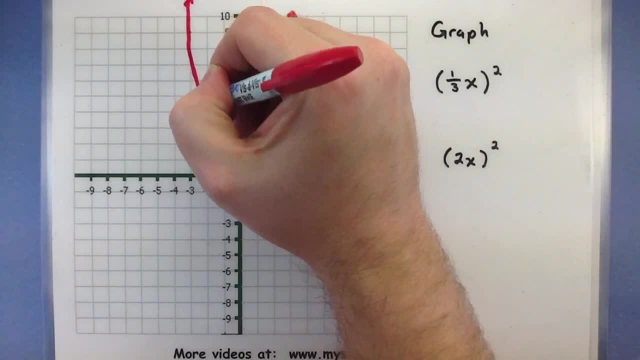 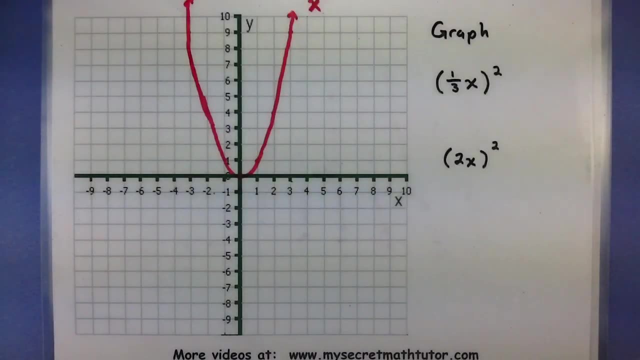 all right, so this guy is our x squared now. both these transformations here are on the inside, so we're going to affect things horizontally. let's start with the first one. this one says one-third x on the inside, and since that number is between zero and one, this will actually stretch it. so keep note that, since we're 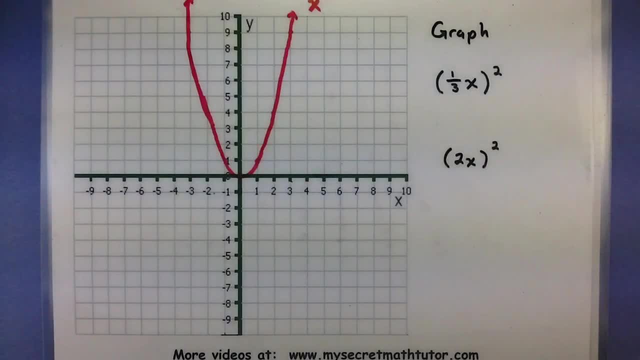 working on the inside. things are working with how many units areoku, expdi momentum. this is displayed right here. so if I go over to number 11, I can working the opposite as what we think they should Now to figure out where we need to put our new points. we're actually going to take all 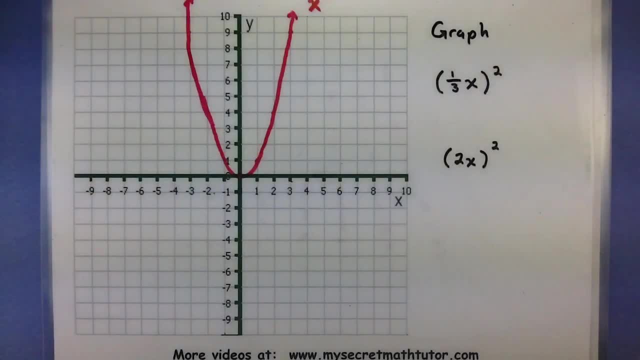 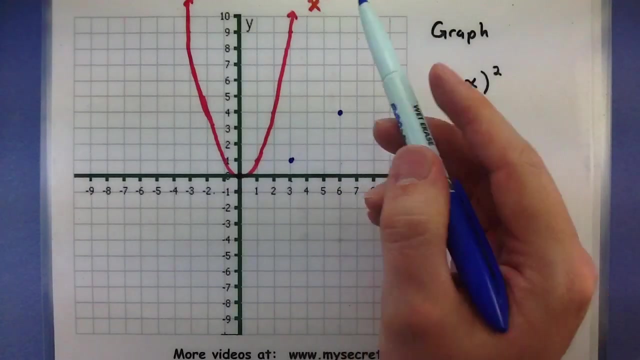 of our x values and multiply them by 3.. So the x value here is 0,. 0 multiplied by 3 is 0.. The x value here is at 1 multiplied by 3, now at 3.. X value here is at 2 multiplied by 3, we'll move it all the way out to 6, and the last. 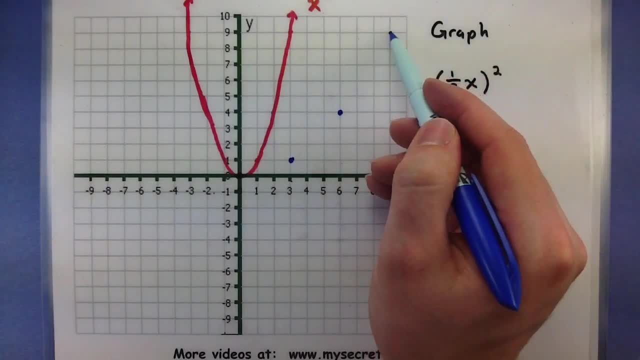 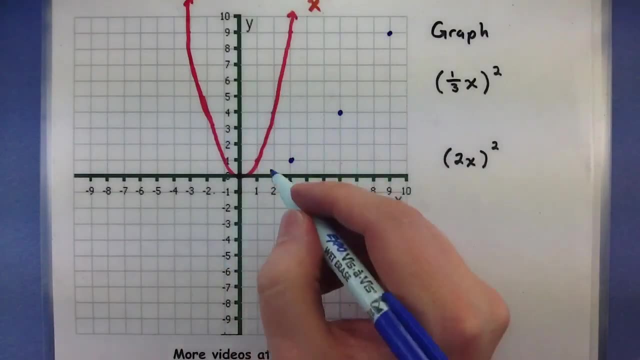 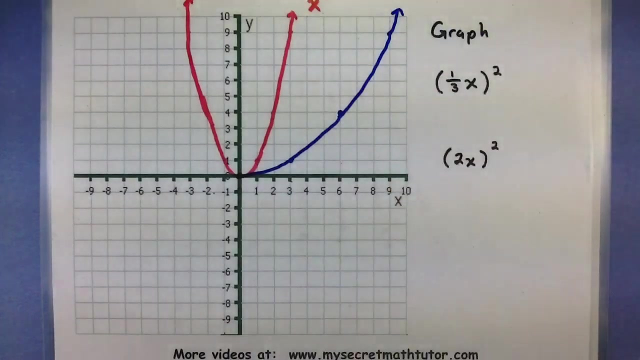 one up here, x value is at 3, this will move it all the way out at 9.. So each x value has been multiplied by 3 and put out into its appropriate spot. So here's half of our new function. looks like a much wider parabola than before. 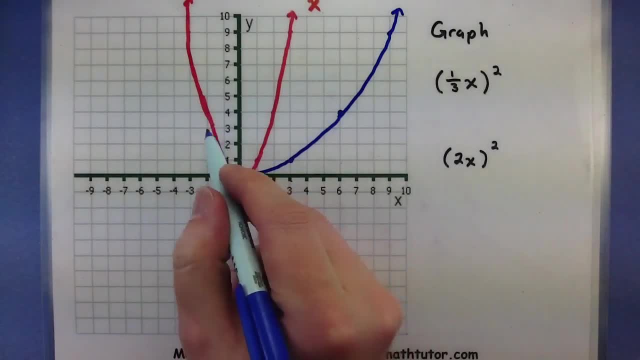 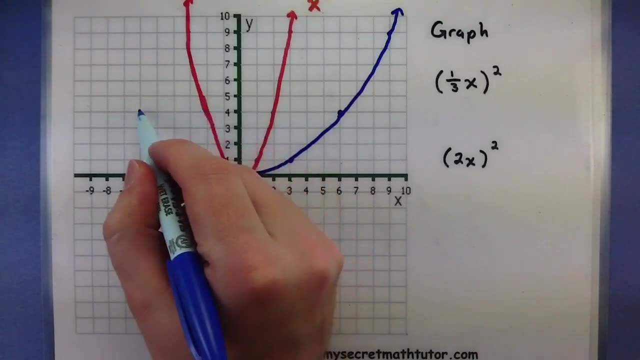 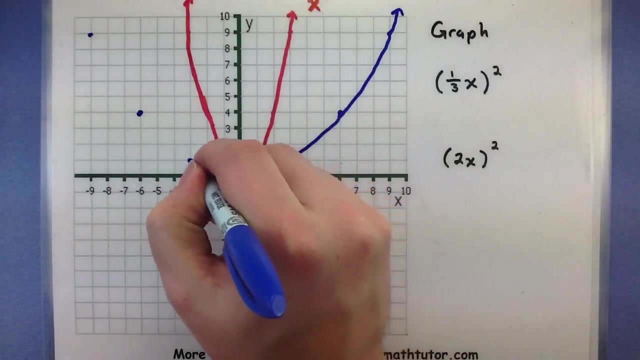 We can do the same things with the x values on the other side. So here's an x value at negative 1.. Now it's at negative 3.. X value at negative 2,, now it's at negative 6.. X value at negative 3,, now it's at negative 9, and there's the other half of our parabola. 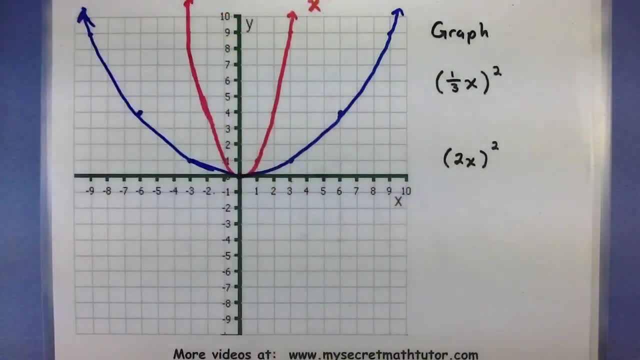 All right, so let's do the other one. This one is 2x quantity squared, so I'm multiplying on the inside by 2, and that's a number larger than 1.. All right, So this will shrink it by a factor of 2.. 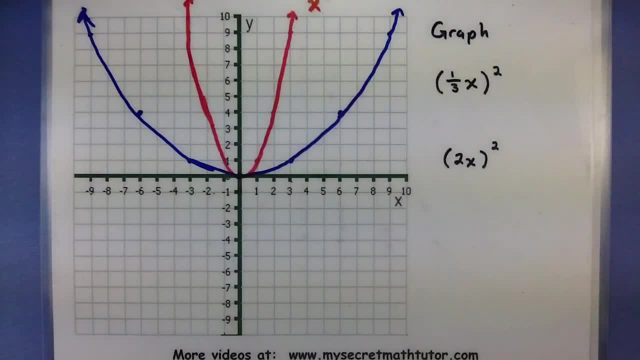 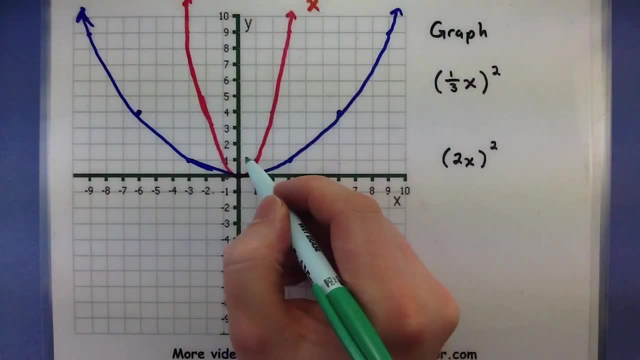 That means we'll take every single x value and we'll actually divide it by 2.. So 0 divided by 2 is at 0.. The x value here is at 1, divided by 2, we'll put that at 1 half. 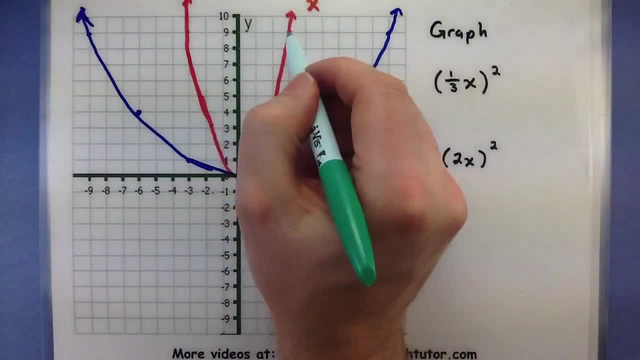 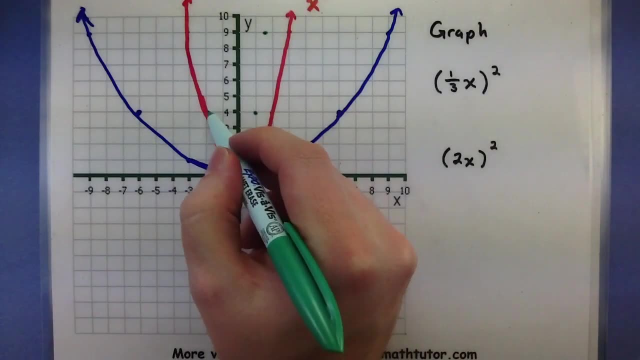 X value here is at 2, moving it to 1, and the x value here is at 3, that is going to be at 1 and 1 half. All right, Do the same thing with the points on the other side. 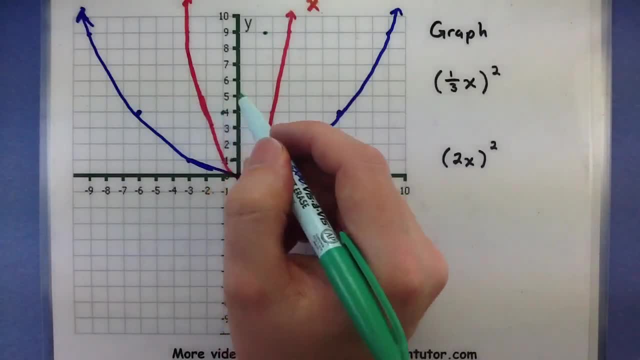 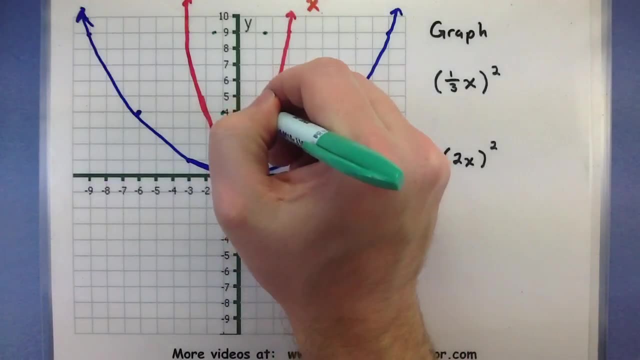 So: negative 2, chop it in half. Negative 3, chop it in half. Now we have some good key points and we can draw out our new transformed function. This one still looks like a parabola, but it's a lot more narrower than the parent function.